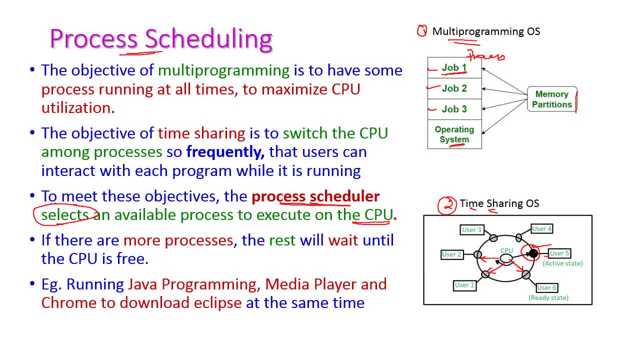 the process scheduler will select the process which is available or which is ready and that will be given to CPU for execution. if more number of process, then the remaining process will wait until the CPU is free. so this is called as process scheduling. let us see one example for this here. I am going 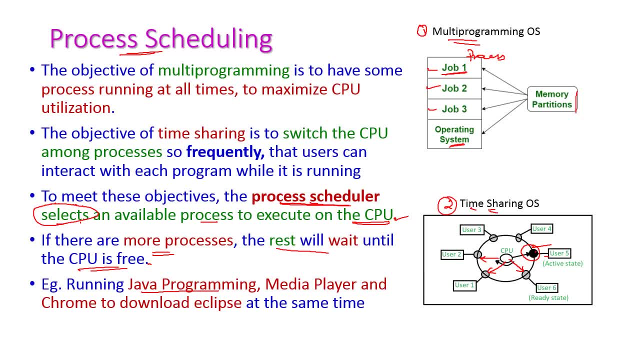 to execute the Java program. that is, I am going to try write the Java program by using Notebook. okay, and I am going to execute this Java program also, and simultaneously I can hear the song, audio song, audio song by using the media player and simultaneously I am going to download the Eclipse. 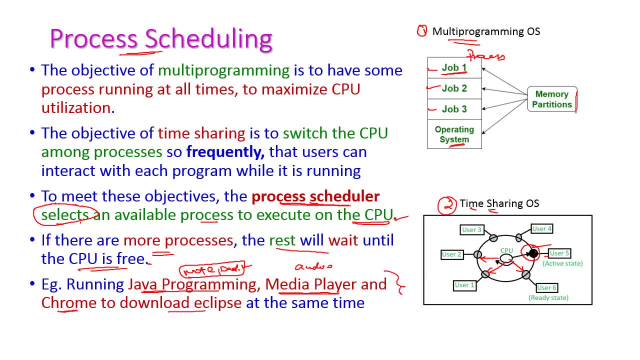 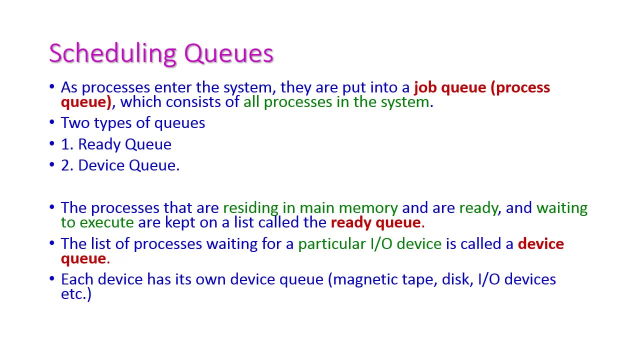 by using the Chrome. and all these jobs will run simultaneously by the CPU without any interrupt of any of the program. and next the scheduling queues. when process enters into the system, then the process will put into the queue, which queue is called as job queue or process queue. this 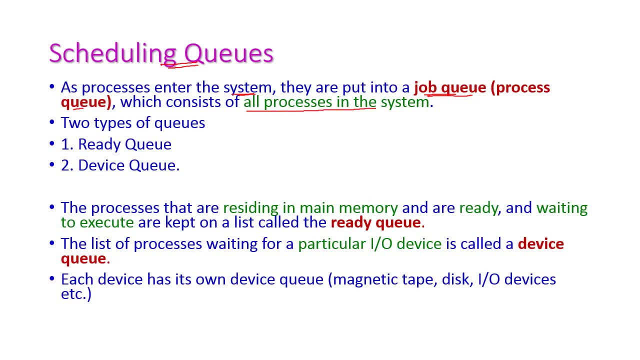 queue consists of all process in the system okay, and they are ready to execute on the CPU and the. there are two types of queues. first one is ready queue and second one is device queue. first let us see what is ready queue. okay, here a process that are residing in main memory. 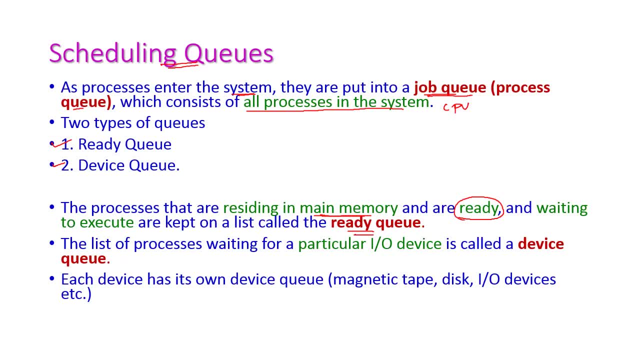 and are ready and waiting to execute, which will keep kept in a list. that list is called as ready queue. that is, if we create a process that is new process, once the process got created, then that process will be executed and the process will be executed and the process will be executed. 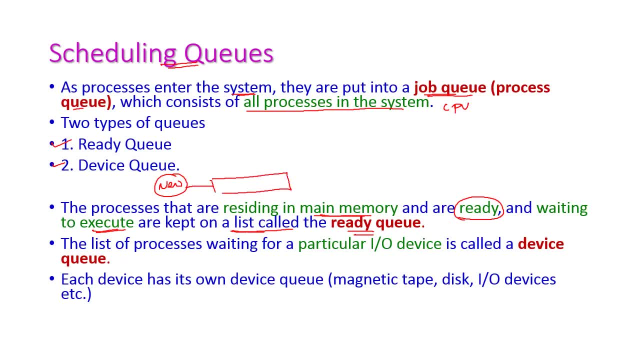 that will be waiting in a queue for executing the executing on the CPU, okay, and this particular queue is called as ready queue. and next one is a list of process waiting for particular IO devices. okay, some process may require some IO devices and that will be wait in a queue. that queue is called as: 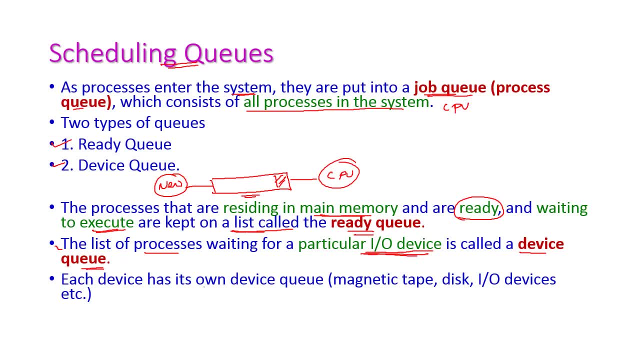 device queue and each device has its own device queue, for example magnetic tape, that is, some process may require magnetic tape and all those process will wait in a queue. that queue is called as tape queue, magnetic tape queue, likewise disk queue, IO device queue, etc. so many device queues. 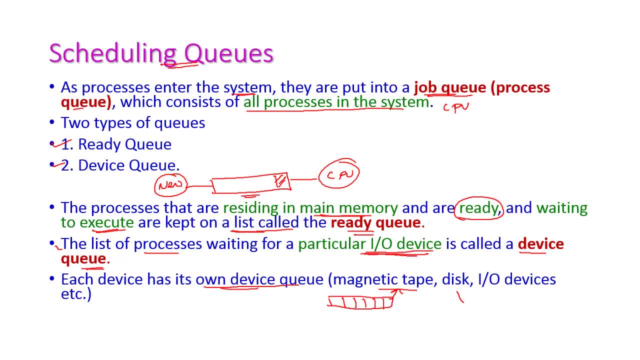 are there. so we are having two types of queues. first one is ready queue and device queue. ready queue is a queue which is ready to execute in the CPU that will be waiting in the ready queue, and device queue used to access those particular devices that will be waiting in corresponding. 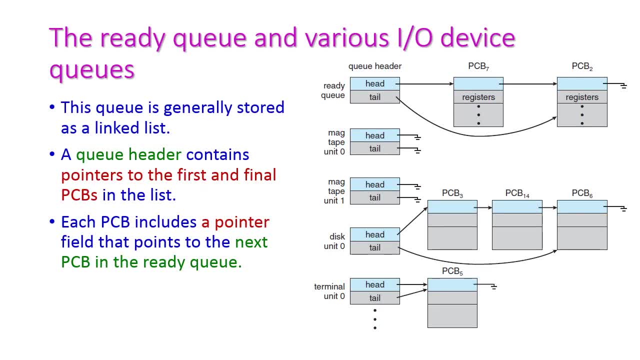 device queue. okay, and here this diagram explains the ready queue and all the other device queues. here the queue is generally stored in a linked list, okay, so in a linked list for all the queue there is a queue header. queue header contains two pointers. first one is head header point, and 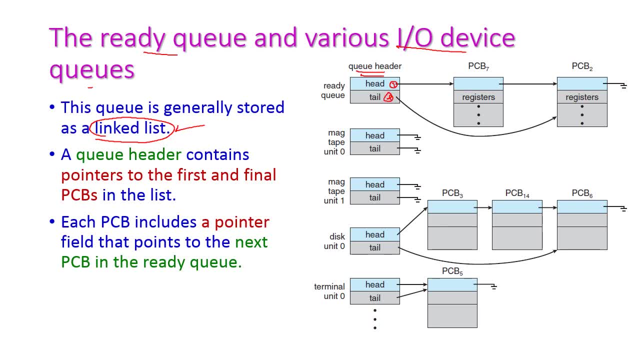 second one is tail: point head and tail. okay, here the queue head contains pointers to first and final PCB in the list. PCB means process control block, isn't it okay? so the head will indicate the first PCB and tail will indicate the last PCB of this particular list. okay, and first one is ready queue. ready queue means the process is ready to. 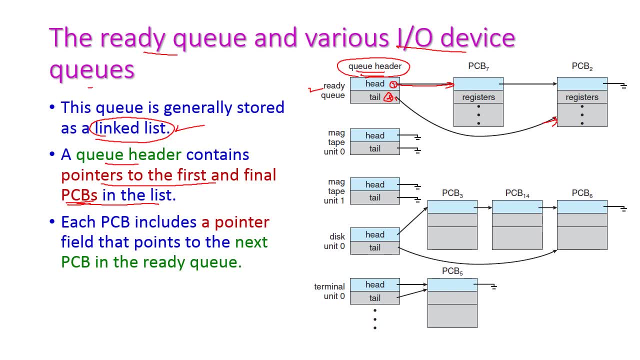 execute in the CPU. that is ready queue and the remaining are device queues and all the other queues are device queues. okay, here we are having magnetic tape queue in the magnetic tape queue. there is no process, is waiting. so all this will be pointing to nothing. okay, magnetic tape, magnetic tape, one unit, two unit, both units. there is no process. when come to disk unit- see here, three process are waiting to access this particular disk: zero unit, okay. so all these will be pointing to nothing. okay, magnetic tape, magnetic tape, one unit, two unit, both units. there is no process. when come to disk unit- see here, three process are waiting to access this particular disk: zero unit, okay. so all these will be pointing to nothing. okay, magnetic tape, magnetic tape, one unit, two unit, both units. there is no process. when come to disk unit- see here: three process are waiting to access this particular disk: zero unit, okay, so all these will be pointing to nothing. okay, magnetic tape, magnetic tape, one unit, two unit, both units. there is no process. when come to disk unit- see here, three process are waiting to access this particular disk: zero unit, okay. so all these will be pointing to nothing. okay, magnetic tape, magnetic tape, one unit, two unit. okay, magnetic tape. one unit. two units. okay, magnetic tape. one unit. two units. okay, magnetic tape. 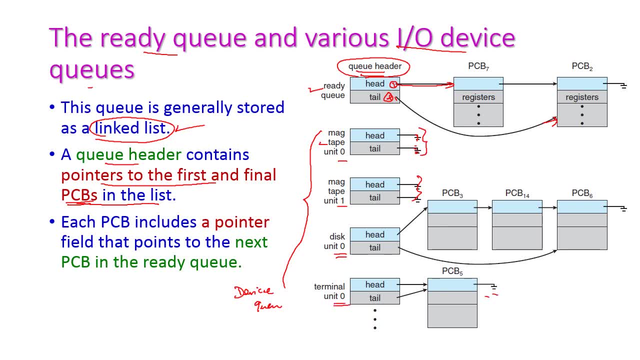 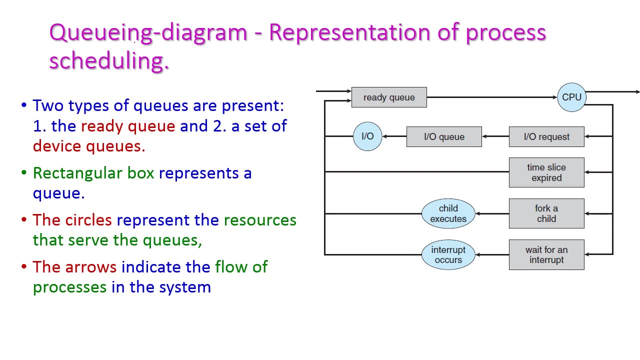 and terminal unit. only one PCB is there, That is, only one process is there. For every process, corresponding PCB is there to maintain all the details. And this is the very important queuing diagram, representation of process scheduling. Here we are having two types of queues. First one is ready queue and second one is a set of 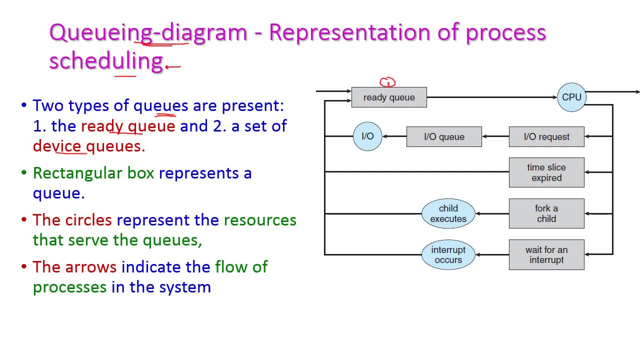 device queues. So this is the ready queue and all the other queues are a set of device queues. Okay, In this diagram, the rectangular box represent the queue. Okay, Rectangular box. So this is the ready queue and all the other device queues are also represent in 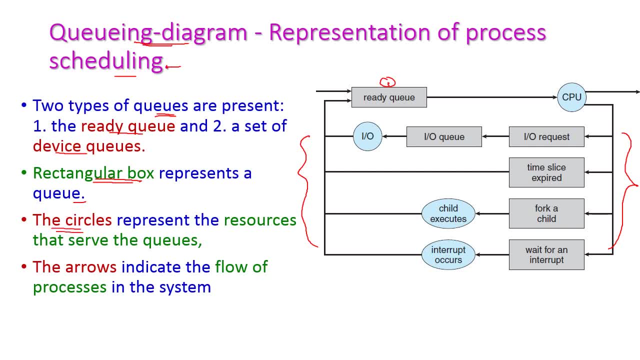 a rectangle and the circle represent the resources that serves the queues. Okay, Here the circle represent the CPU and this is I-O devices and child needs to be execute and interrupt occurs. Okay, So it gives the resources and arrow which indicate flow of process in the system in which. 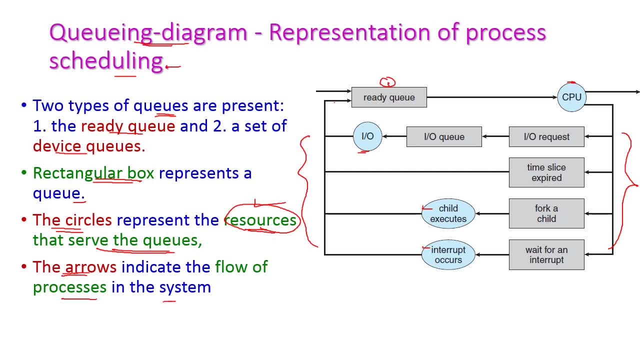 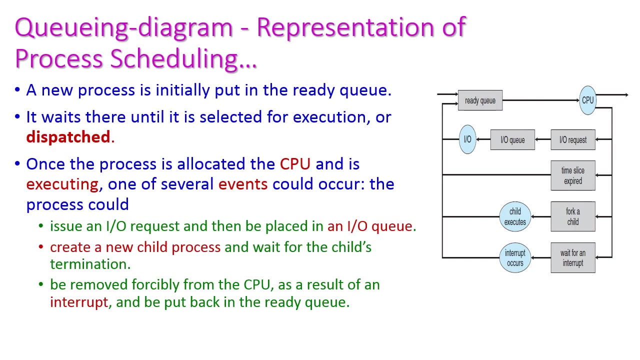 direction the process will be flowed. Okay. So the arrow indicates this is new process will be given to ready queue And then that process will be given to CPU. So arrow represent the flow process. When new process created, say new process created, then the process will wait in the ready queue Once the process got a dispatched. 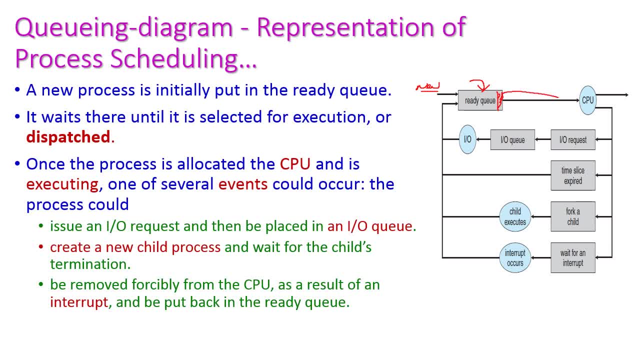 dispatched by the scheduler. then the process will access the CPU for execution. Okay, While executing this CPU, many events may be occurred. First the process may request an I-O devices for execution. further execution- then that will wait in the I-O queue. 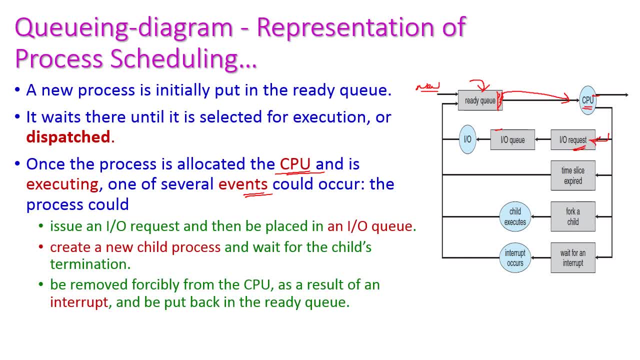 Corresponding I-O queue, Then it will go back to the ready queue. Otherwise, is there is time slice expire, then automatically that will go back to ready queue and sometimes it may create a new child process, Thenaniu morning time process by calling the fork function okay, then the process will be terminated. 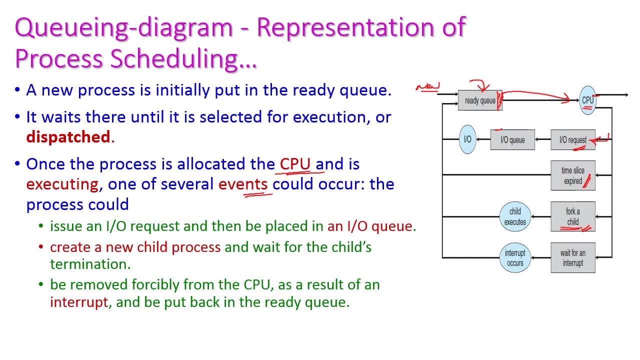 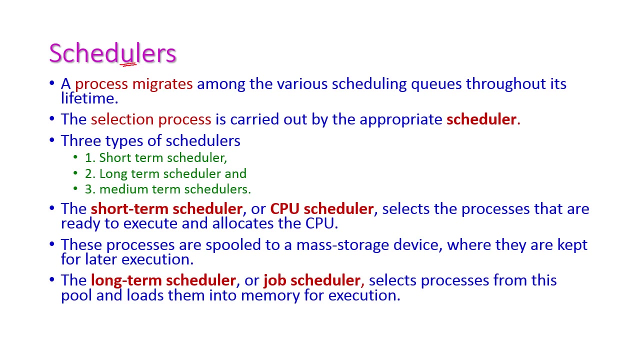 until the child got executed right. and other one is the. in is suppose if any interrupt occurs then the process forcibly exit from the CPU and that will go back to ready queue. the next one is scheduler. so in the process of process execution it will migrate among various scheduling queues throughout this. 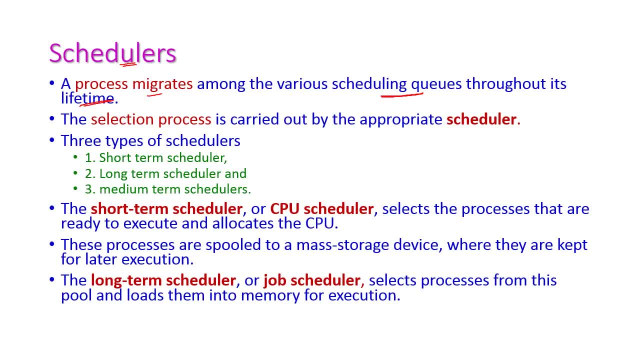 lifetime and the process selection will be carried out by the scheduler. okay, in each queue, the process will be selected for the next pura purpose, isn't it? so the selection will be carried out by the scheduler. Here we are having three types of scheduler. First one is short term scheduler. 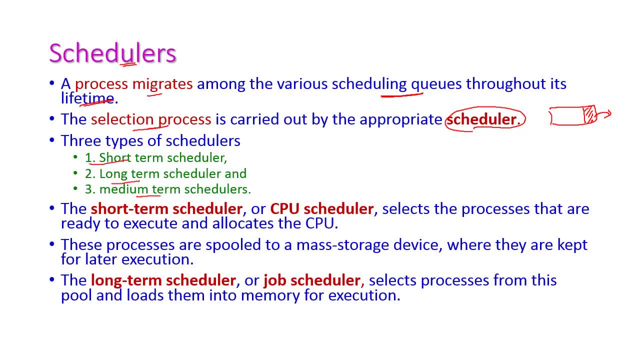 and long term scheduler. Next one is medium term scheduler. The short term scheduler is otherwise called a CPU scheduler because the CPU will execute more number of process at a time. that is very often. the scheduler will assign the process to the CPU Because the process are in ready queue. 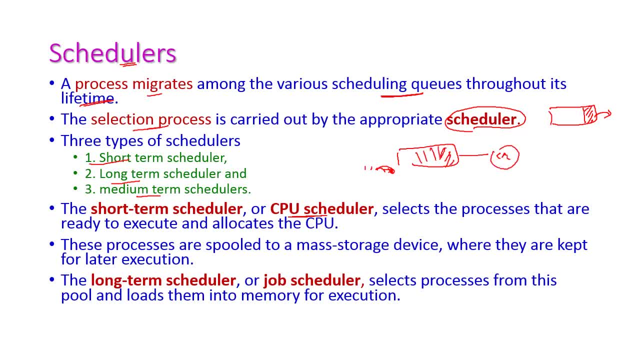 and the CPU is here, the scheduler will very often, very frequently, assign the process to the CPU. hence it is short term scheduler. And when come to long term scheduler, all the other schedulers, that is, other than ready queue scheduler, are called as long term scheduler, that is, device scheduler. 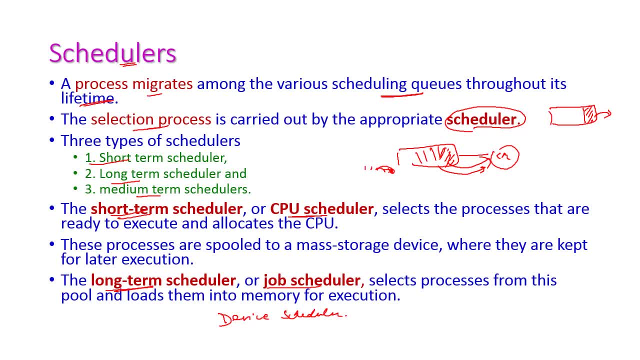 The long term scheduler is otherwise called a CPU scheduler, because the CPU is in ready queue. The long term scheduler is also called as job scheduler. Why? Because the scheduling will be taken place only after completion of first process. If one job completed, then only the other job will be. 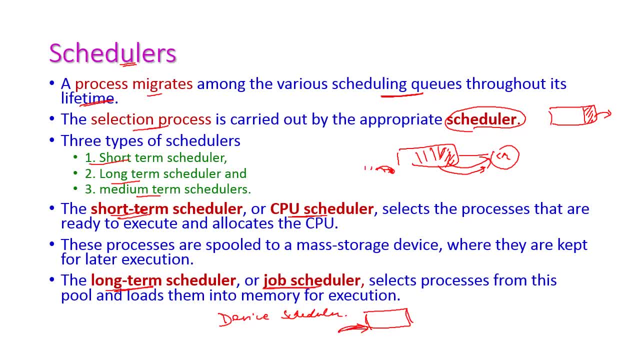 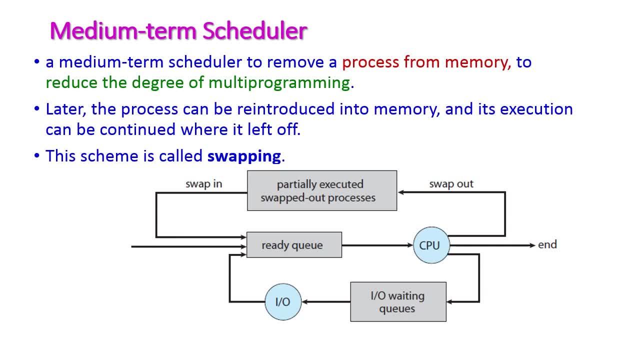 given for execution. Hence it is called as long term scheduler. The next one is medium term scheduler. The modern operating systems will use only this medium term scheduler. In this scheduler it will remove the process from the memory, that is, from the main memory, to reduce the degree of